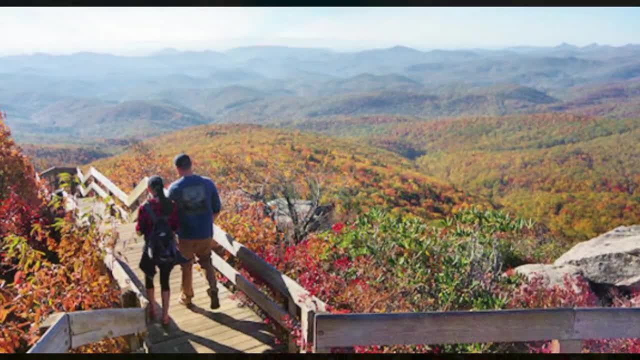 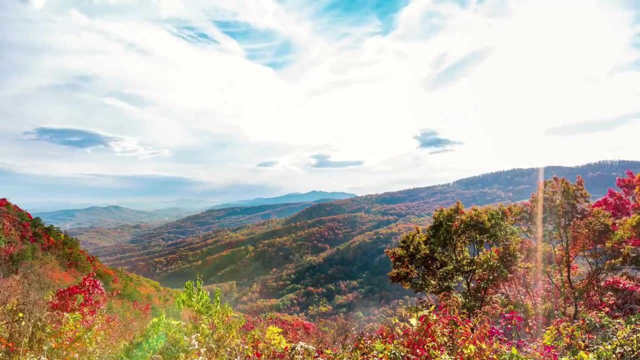 From Asheville's famous Blue Ridge Mountains to Winston-Salem's renowned festivals, there is something for everyone to enjoy in North Carolina. For those looking to make a new home in the South, North Carolina is an ideal choice, with plenty of reasons why you should choose it. 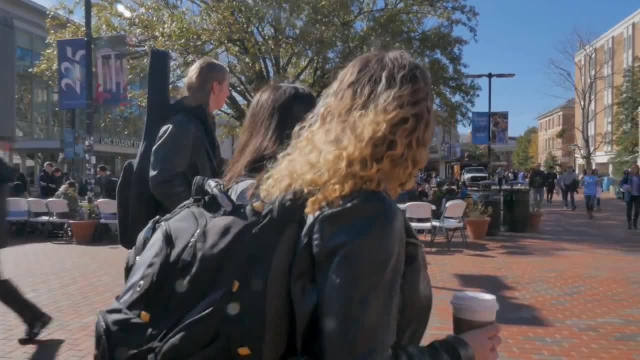 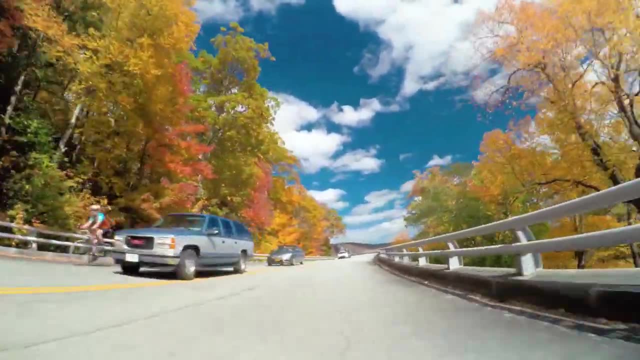 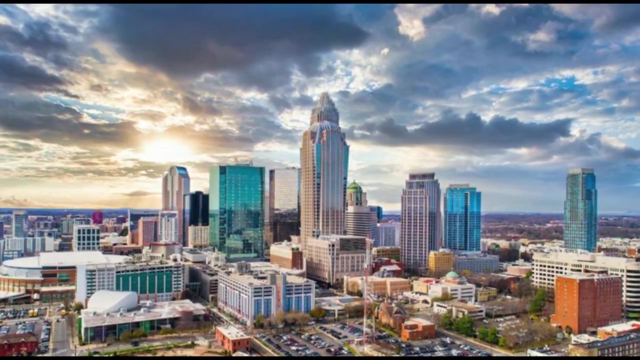 From stunning natural beauty to abundant educational opportunities, cultural attractions, north carolina has something to offer everyone. top seven places to live in north carolina. here are the top seven places to live in north carolina. one: charlotte. from healthcare to technology, charlotte is an economic hub in the south with a vibrant nightlife and 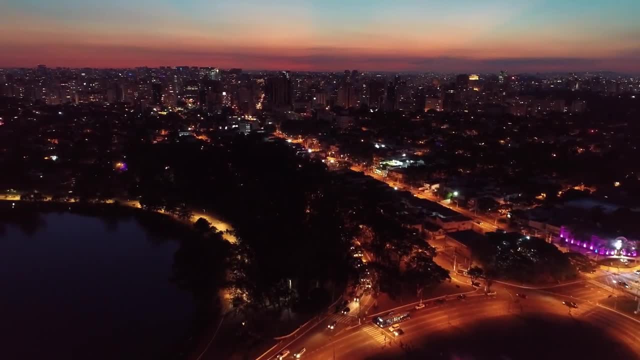 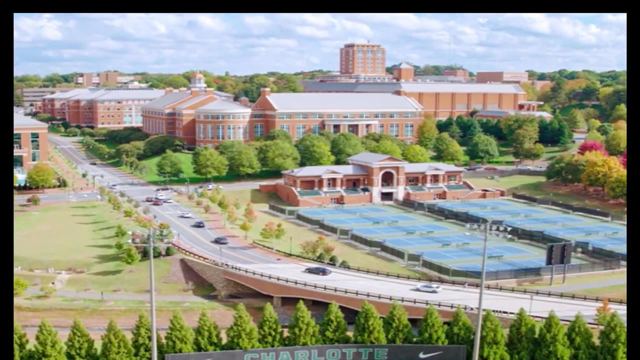 plenty of cultural attractions. it's no wonder why this city is top on the list of places to live in north carolina, also known as the queen city. charlotte is home to the carolina panthers and nascar's hall of fame, so you can enjoy a football game or take a tour of the museum. dedicated to american motorsports. now, when it comes to housing and expenses, it might be a higher price tag than most, but with all the benefits that come with it, you get your money's worth. being one of the top cities in north carolina, charlotte is a great place to live. 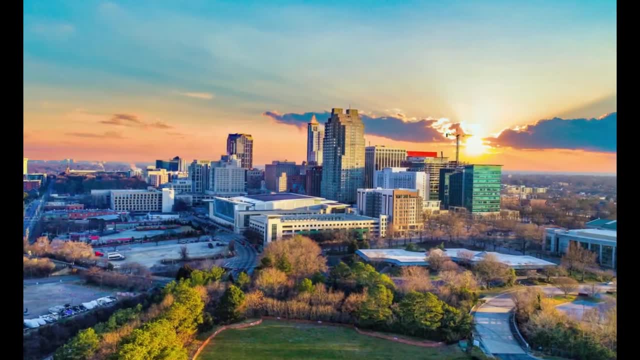 2. raleigh- right after charlotte is raleigh. the state capital of north carolina is north carolina. charlotte is a great place to live. two raleigh- right after charlotte is raleigh. the state capital of north carolina is north carolina. 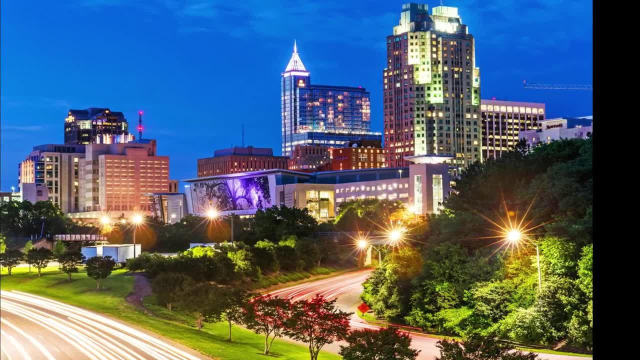 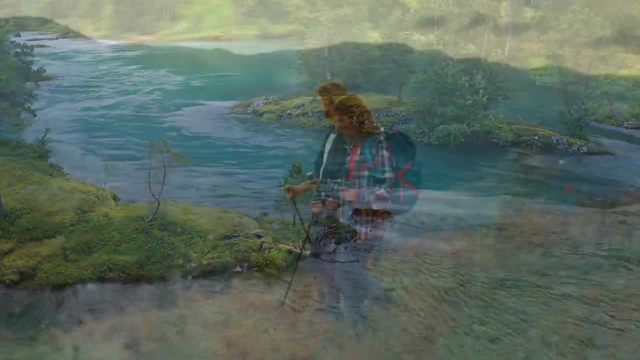 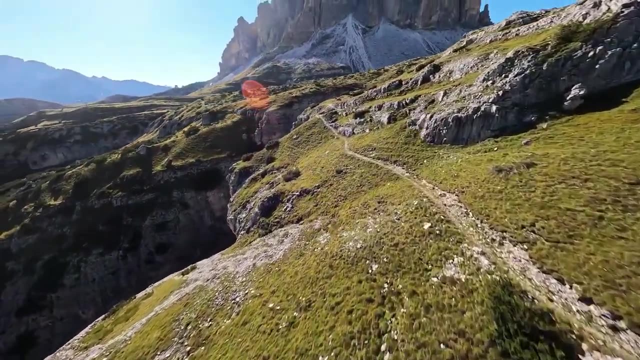 north carolina. this beautiful city is filled with plenty of history, culture and natural landscapes. the city provides you with all the amenities needed while being surrounded by nature, such as lakes, hiking trails and other outdoor recreational activities. known to be one of the fastest growing cities in north carolina, you can enjoy many retail and dining options in the area. 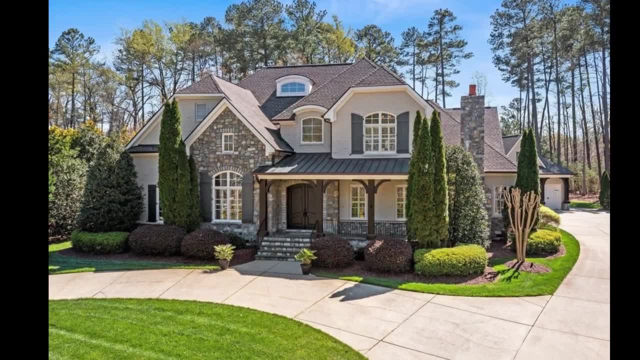 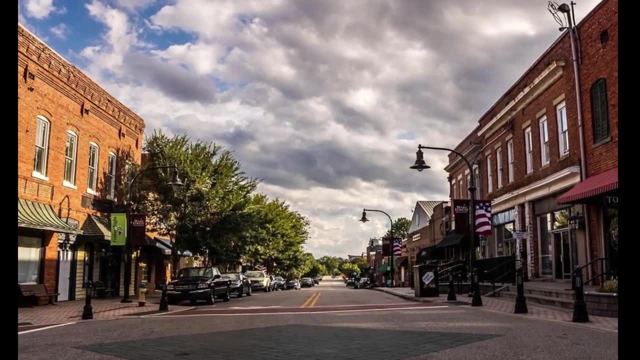 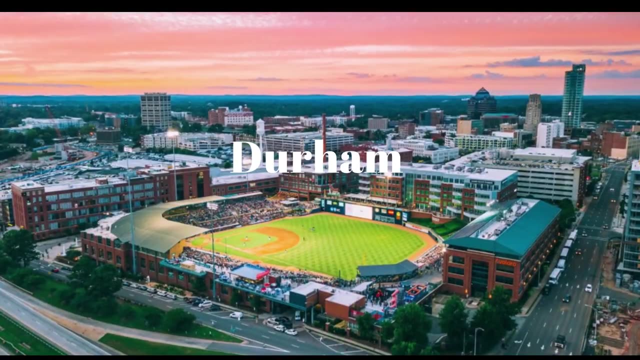 when it comes to housing, raleigh has a higher median home price than charlotte, but still provides you with plenty of different options. so when searching for a place to live in north carolina, raleigh should be high on your list. durham known as the city of medicine due to its large medical research and healthcare industry. 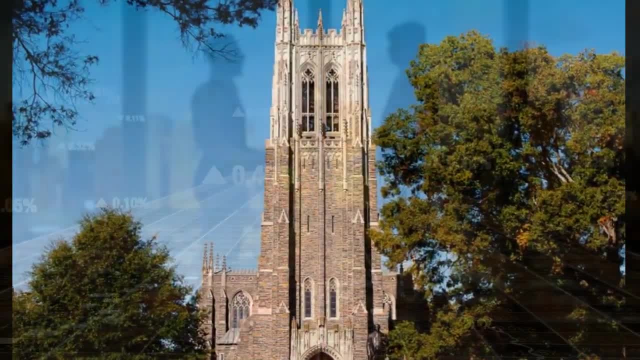 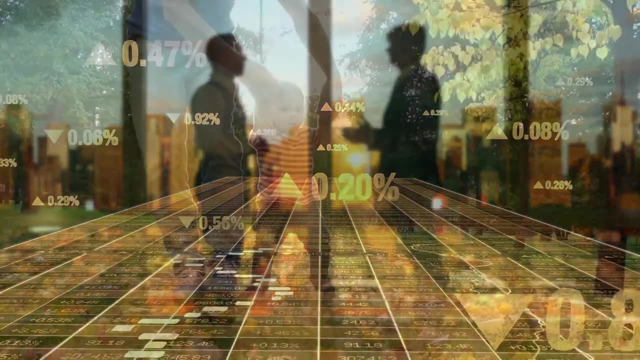 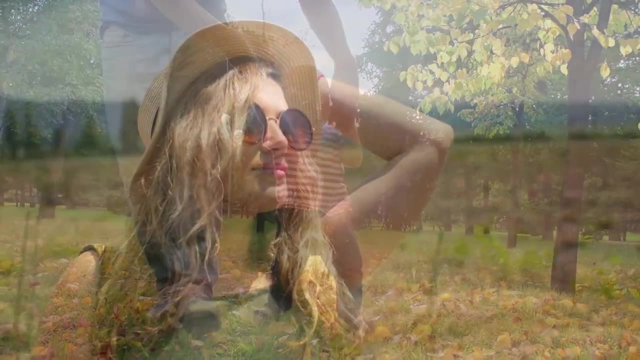 durham is home to duke university, the largest private employer in the city. the city also has a strong economy based on the banking, finance, technology and manufacturing sectors. with an abundance of parks and green spaces, durham offers ample outdoor recreational opportunities for its residents. with its mix of urban and rural attractions, durham is one of the 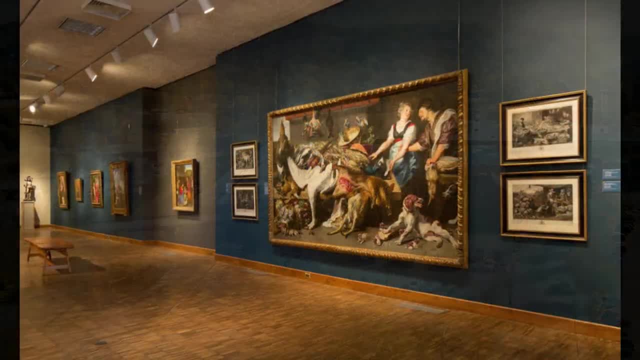 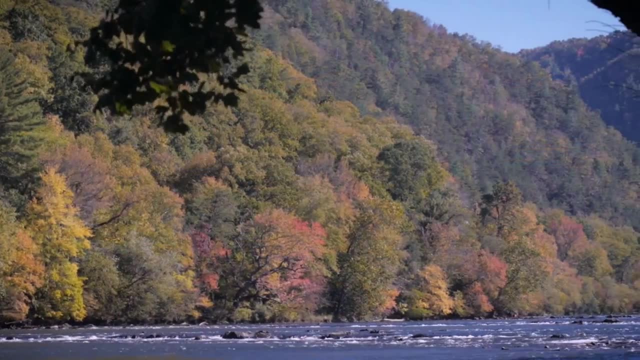 fastest growing cities in north carolina. the city also boasts a vibrant art scene, with numerous art galleries, music venues and performing arts facilities. durham is known for its diverse population and rich cultural heritage. the city offers something for everyone, so you can find a variety of activities to enjoy. 5. winston-salem- winston-salem. winston-salem is another great option for those looking to relocate to north carolina. with its vibrant arts and culture scene, winston-salem offers plenty of attractions and activities for residents to enjoy. the city also boasts a thriving economy, with many 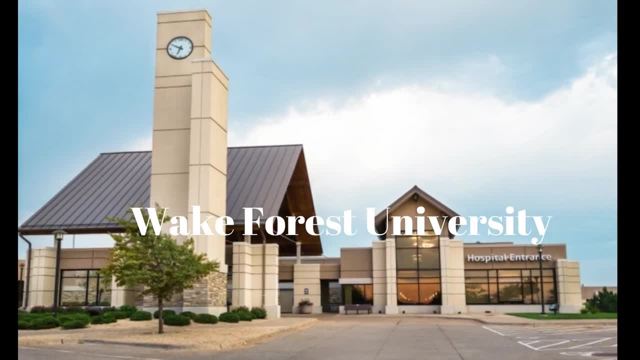 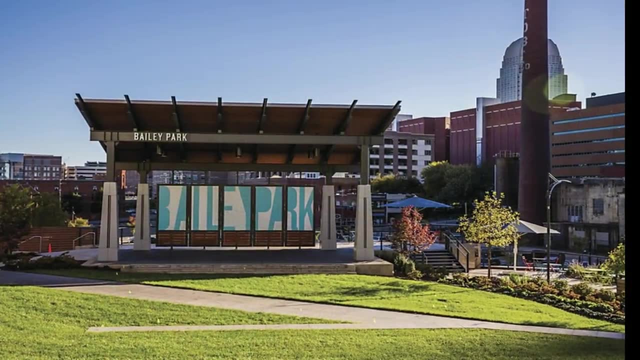 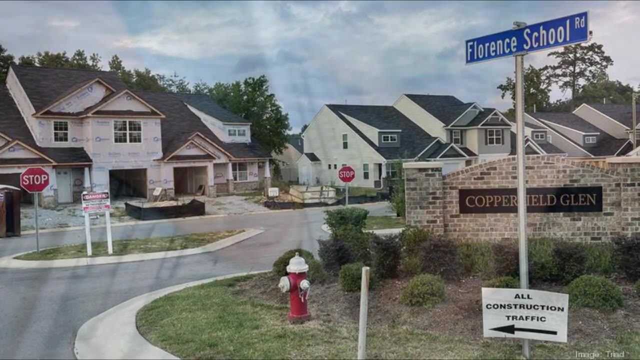 high-profile employers in the area, such as wake forest university and bb t. also, there are several recreational greenways for exercising outdoors. you can unwind at bailey park or enjoy wake forest university sports events. one of the best parts of winston-salem is the cost of living, with an average monthly expense of six thousand dollars. 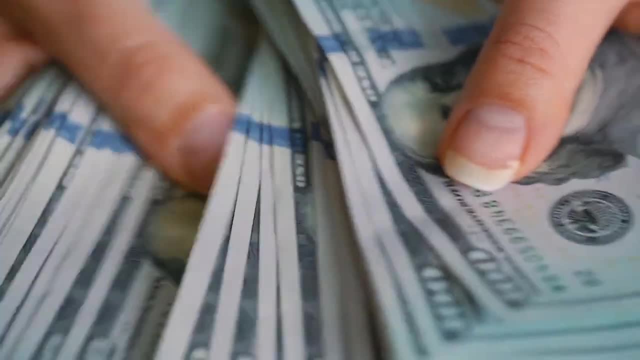 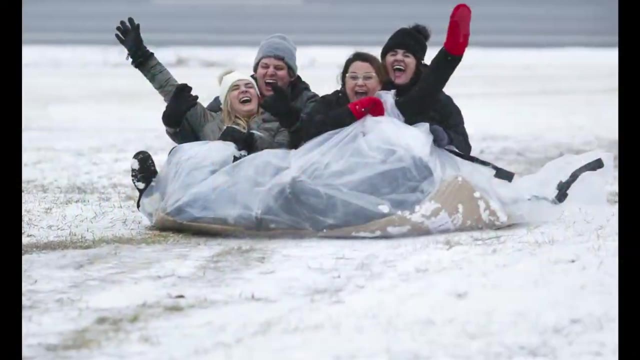 and a median home price of three hundred twenty thousand dollars, it's an incredibly affordable city to settle down in. plus, residents get to experience all four seasons each year, from summer festivals to winter snowfalls. winston-salem is the perfect place to experience all the perks of living in north carolina. 6. asheville. located in the blue ridge mountains of north carolina, with its vibrant and diverse culture, asheville has attracted people from all over the world. the small city is home to many great local businesses, restaurants, bars and breweries that give it an eclectic flair- the biltmore estate and north carolina arboretum also make great opportunities to explore the city. asheville also boasts plenty of outdoor activities such as hiking, camping, biking and skiing, which make it the perfect place for people who love to explore. though, living in asheville is a bit pricier than most north carolina cities, with an average monthly expense of eight thousand. 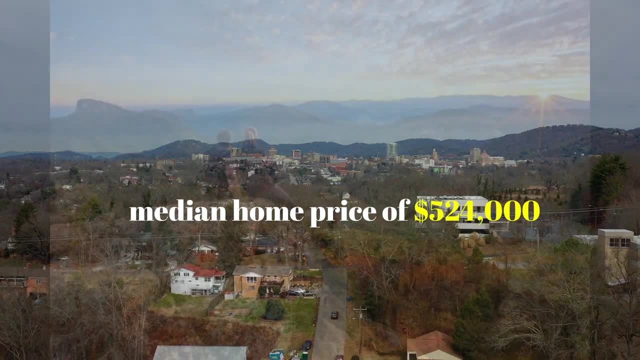 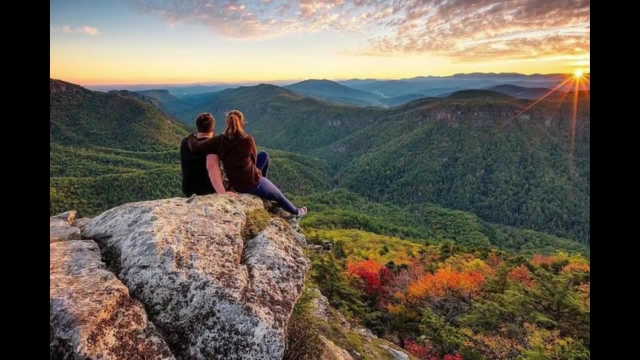 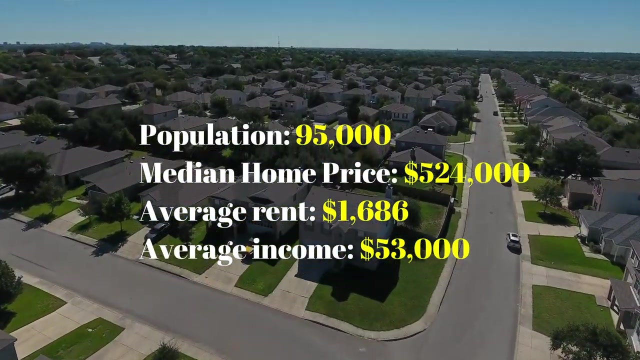 dollars and a median home price of five hundred twenty four thousand dollars. however, residents get their money's worth with the wide variety of attractions and activities, plus the stunning mountain views make it worth every penny 7. wilmington: wilmington is a vibrant city that embraces its colonial port town vibes in quaint. 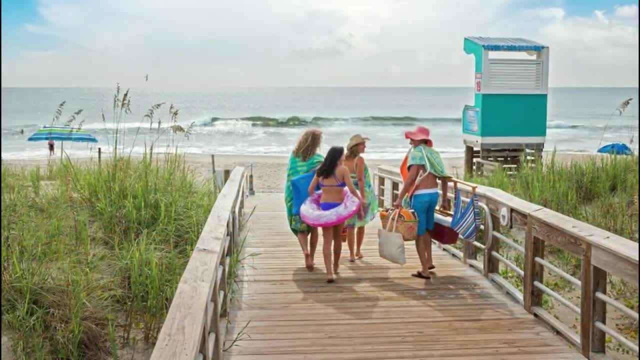 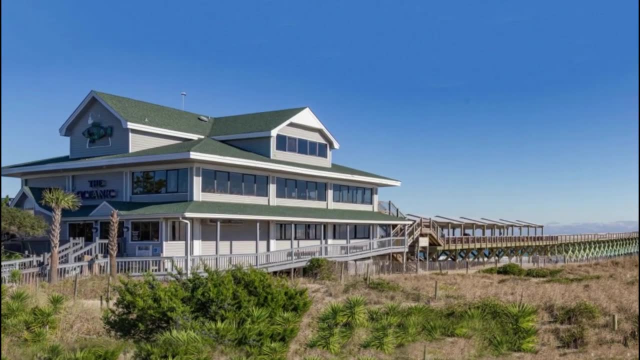 downtown, along the way the Cape Fear River, There are several pristine beaches, like the Wrightsville Beach and Oak Island, that you may enjoy. But that's not all. it continues to expand, with newcomers choosing to make this great place their home. each year, Wilmington is bursting with youthful energy, thanks. to the vast student population of UNC, Wilmington and Cape Fear Community College, as well as a continuous stream of college graduates. Thanks to less population density and a wide variety of housing styles, this coastal city offers some great deals on homes If you're looking for a. 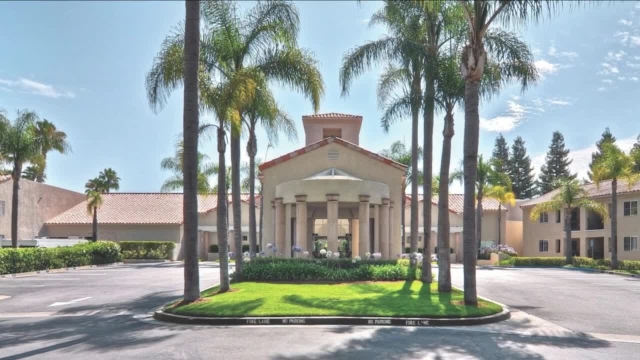 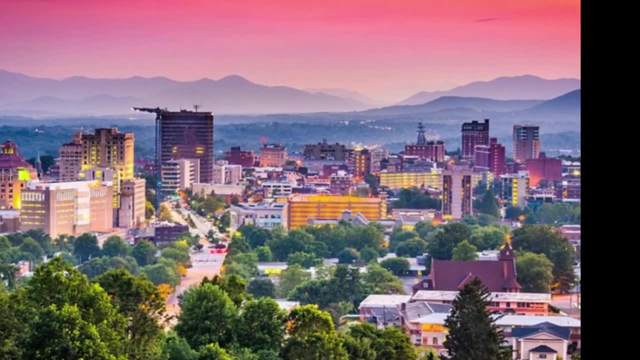 laid-back atmosphere with plenty of activities to engage in, then Wilmington, North Carolina, should be at the top of your list. With so many great cities to choose from, North Carolina is a wonderful place to call home, From bustling metropolitan areas to small mountain towns.